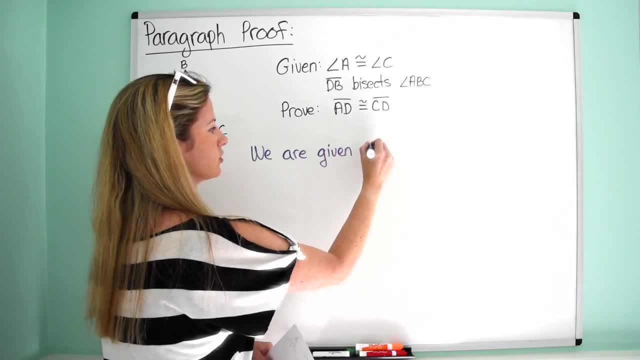 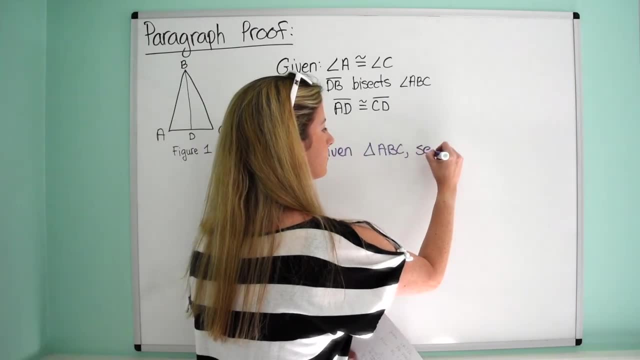 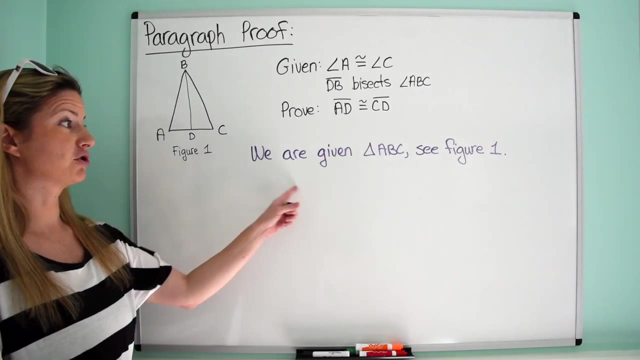 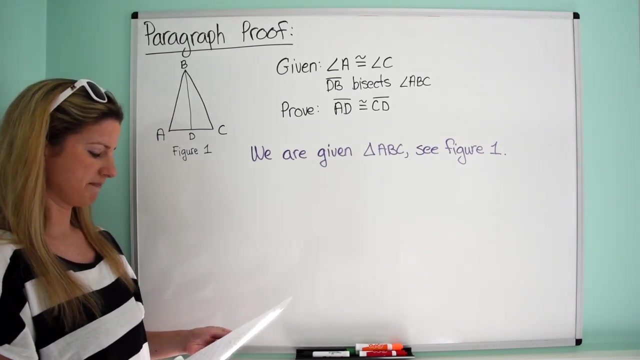 So we're going to start with our given triangle: ABC, um, c, figure one. Okay, now, not every teacher may require that you write that first step. I you know. I think it's good, because then we know what we're talking about. Um, okay, so now the next thing we do for 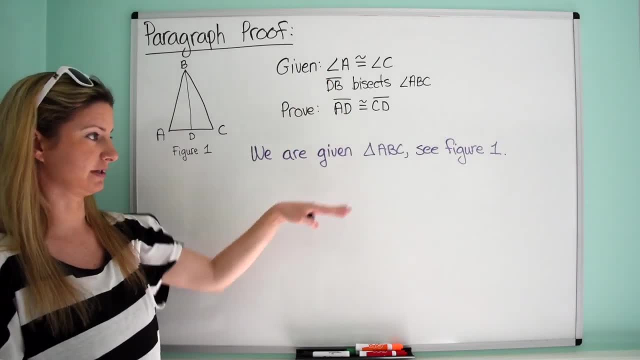 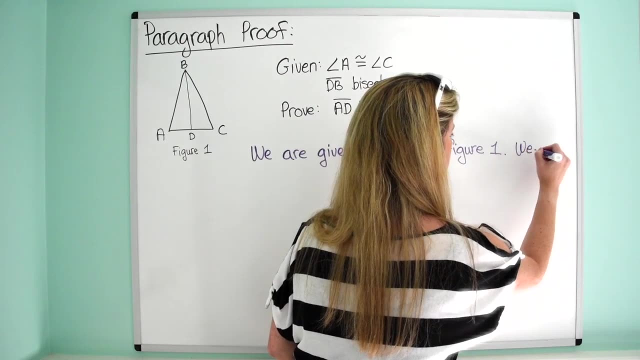 paragraph proof is we list our given. So remember, in our two column form we're going to start with column proof. we just list them, Okay, but in a paragraph proof we have to actually write them out. So we write: we are given that I'm going to come all the way over here. We are given. 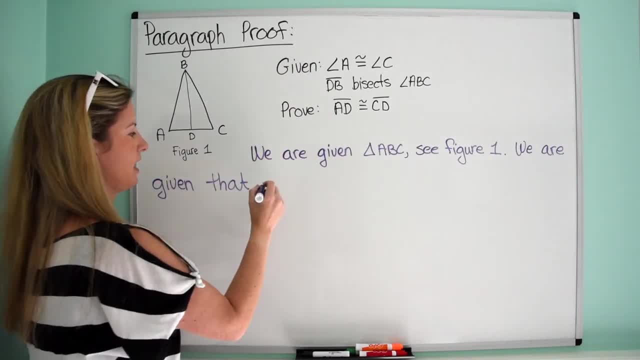 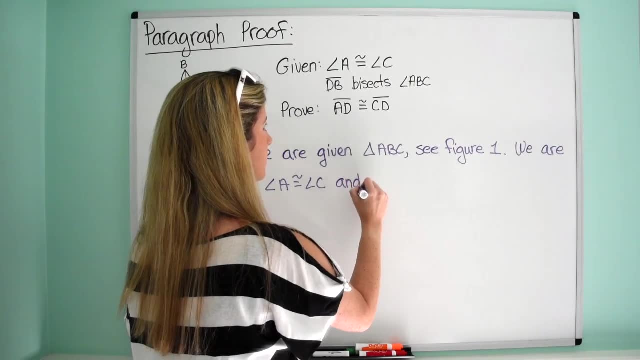 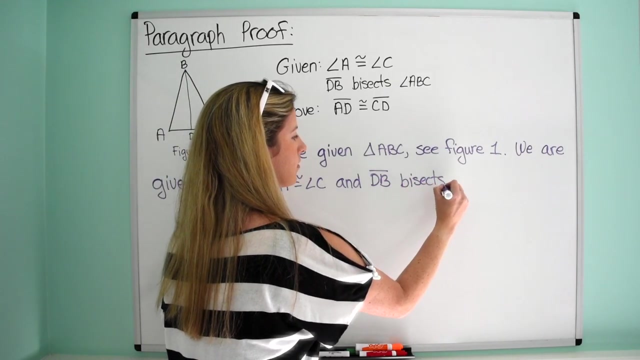 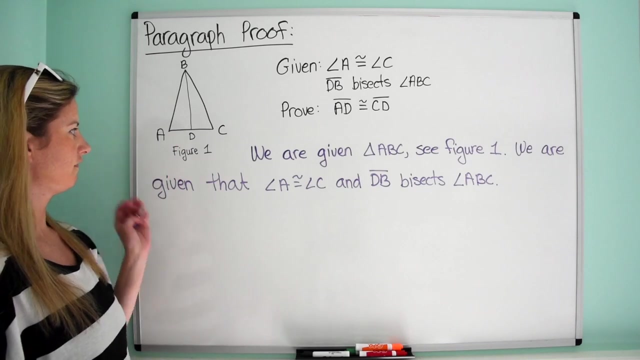 that and then you just write it out: Angle A is congruent to angle C and DB segment DB bisects angle ABC. Perfect, Okay, so we've told everybody what figure to look at. Um, we've now listed our given, So now, 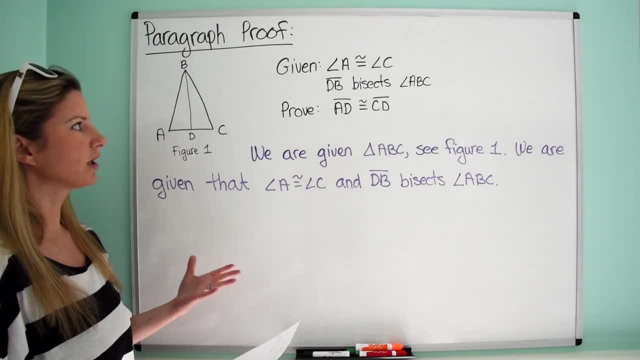 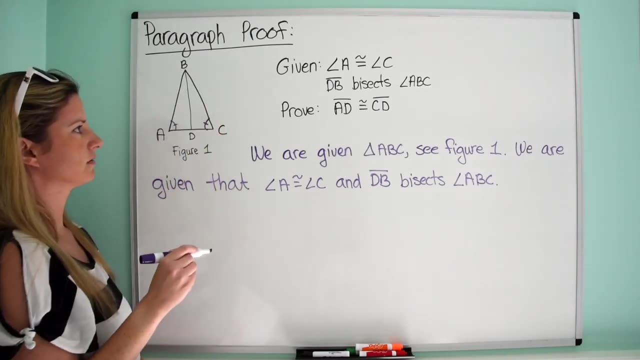 we have to get into the proof, Okay, so what we're going to do here is- I think it's good always to mark off. So we have: A is congruent to C angle A is congruent to, and then DB bisects angle ABC. 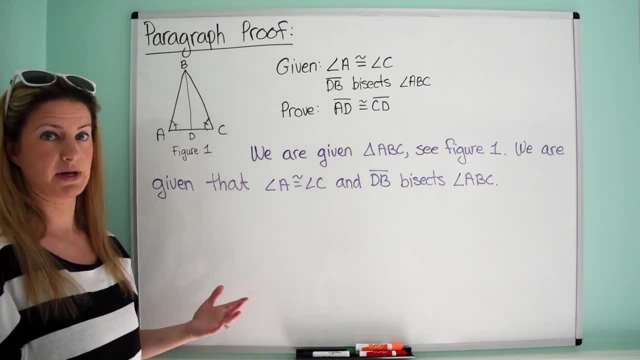 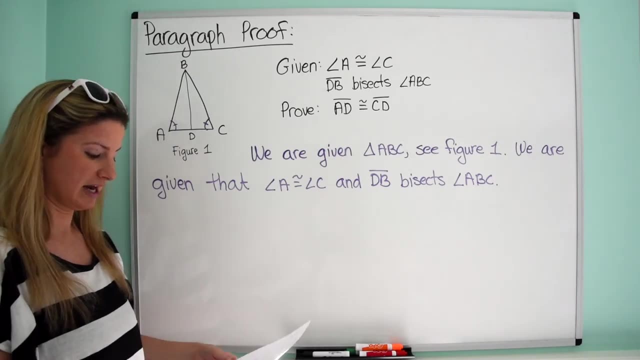 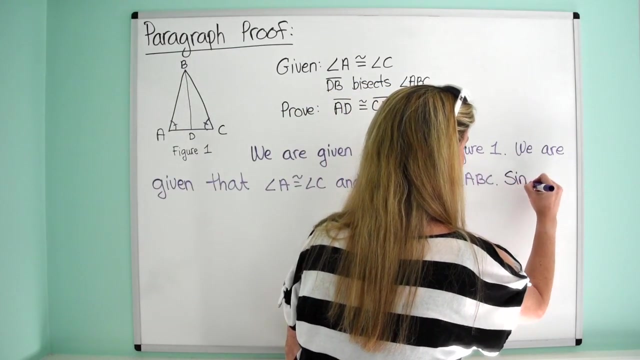 Okay, so when DB bisects angle ABC, what does that mean? Well, we we know that when you have an angle bisector, it's going to split an angle into two congruent angles, So we're just going to write that out. So what we're going to say is: since segment DB bisects ABC, So since segment DB bisects. 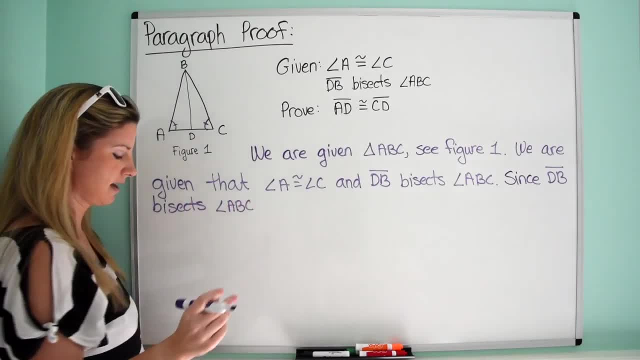 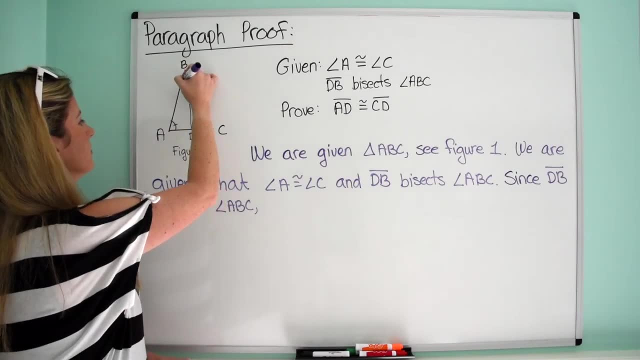 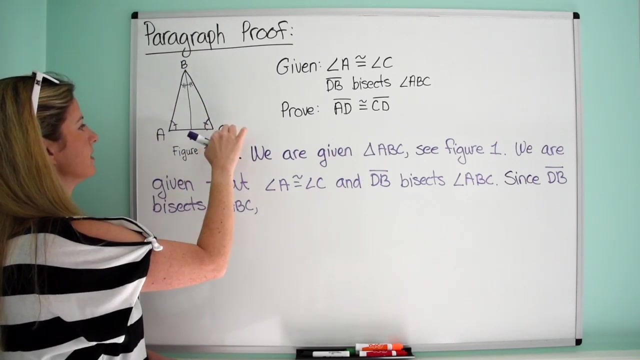 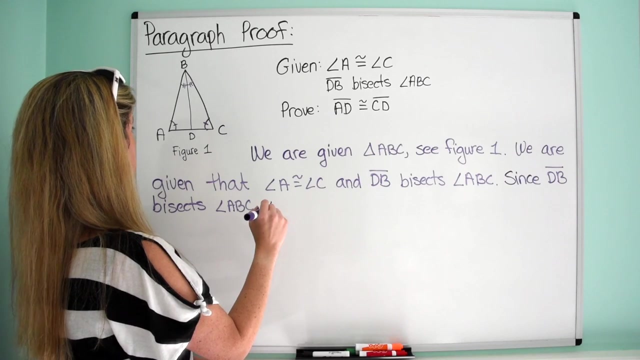 angle ABC. Okay, comma, Okay, um, angle ABD. So this one's going to be- I should put two there- That angle is going to be congruent to this angle. So angle ABD is going to be congruent to angle CBD. Okay, so let me just write angle ABD. 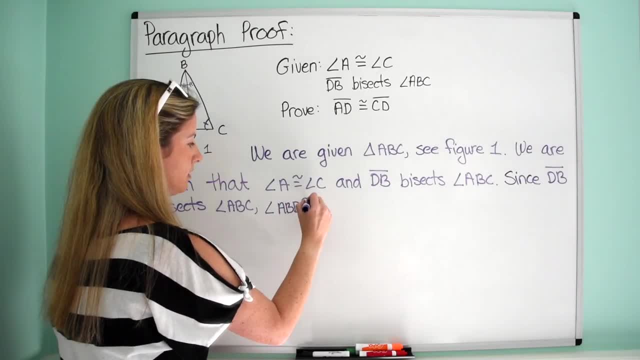 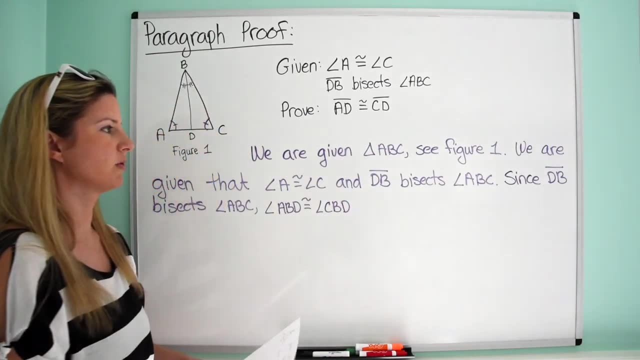 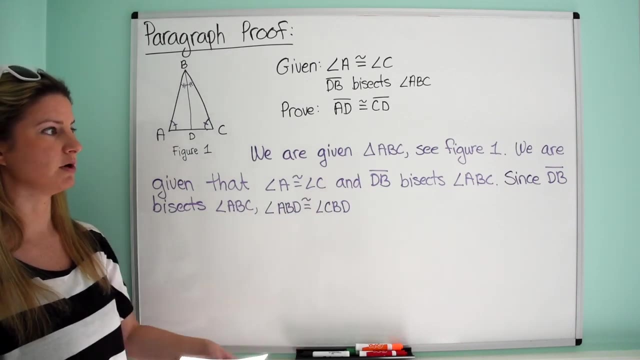 is congruent to angle CBD. Now here is where we have to write that thing. So remember, with your two column proof, you wrote the statement, So you would write the statement. So you would write the statement, So you would write the you know this as your statement, and then your reason would be: um definition of angle bisector. So 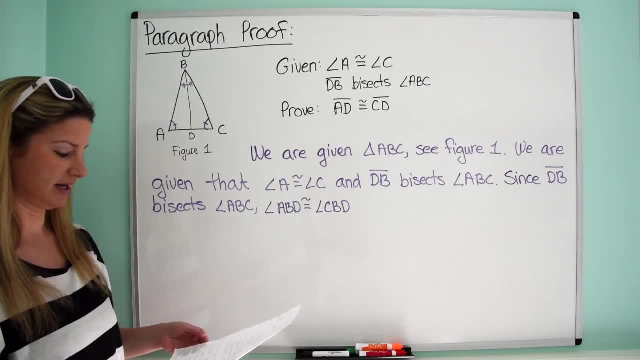 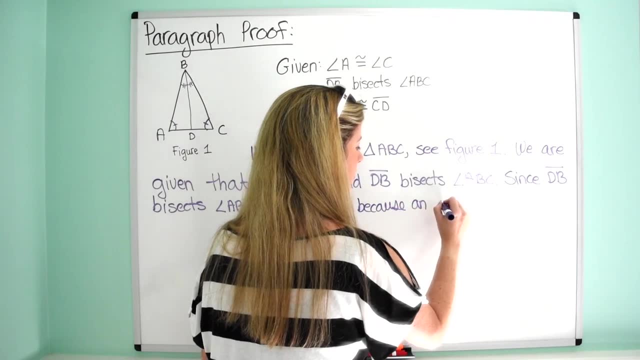 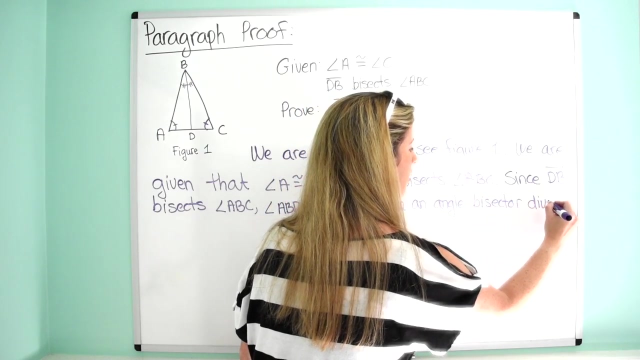 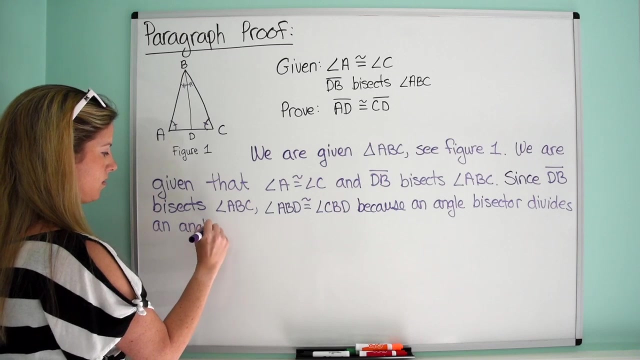 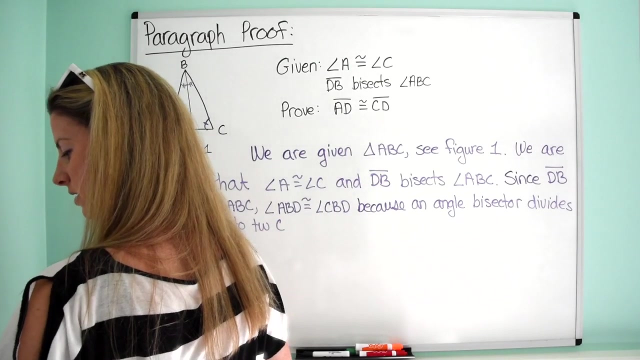 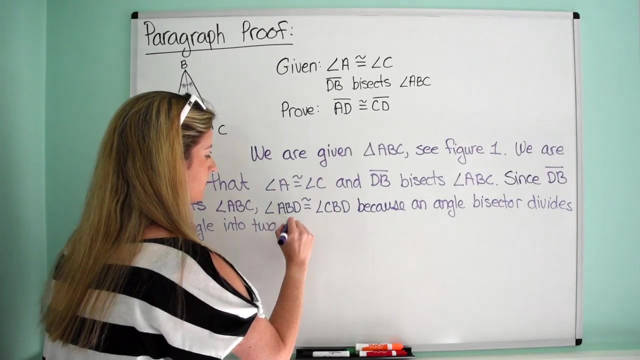 in this case, what you're going to write is because an angle bisector divides an angle into two congruent angles, Just so you can think about your whole thing. So you're going to write this alone, Ok. so since, Ok, three points we got, So here's one: angleотив están. So when you call that one angle, vicex angle. 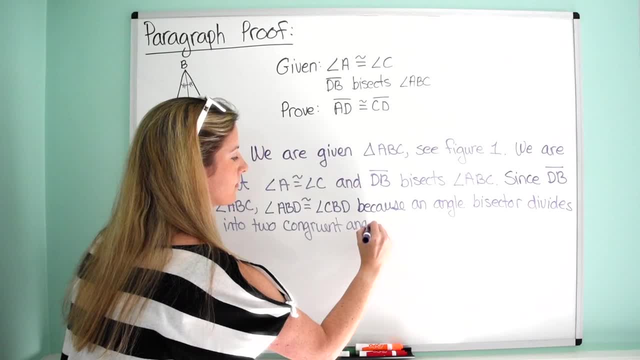 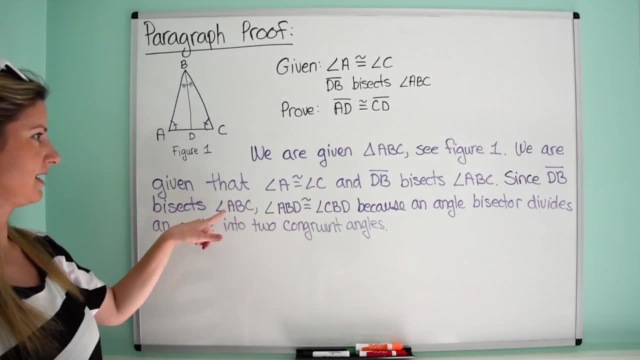 AB3,. Ok, so bottom angle is serving. So B1 angle, AB going to be Griffian. Ok, this angle, Db angle, ABC, This is our angle, This is our level of angle, swarm angle. So let me say for this, T should be 0. Whoops, I got the 0 on 2早 Christi. So since DB bisects angle ABC ibicext angle prologue on submission zero, then let's just write down both angles ABD, and bargain to one angle Aued services. 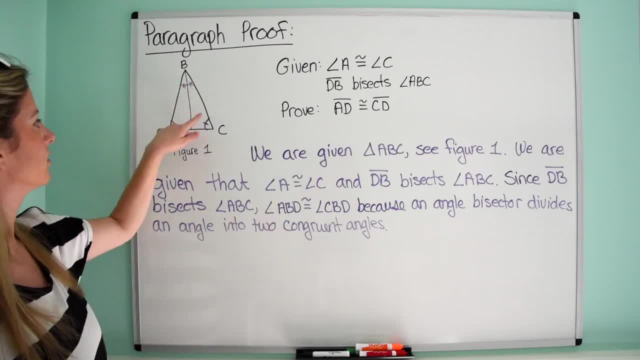 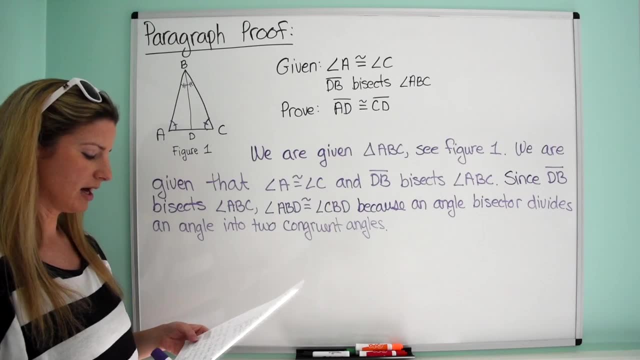 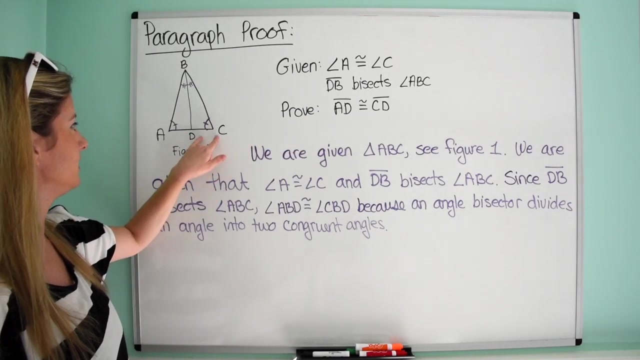 ABC. right up here, We know that ABD is congruent to CBD because an angle bisector divides an angle into two congruent angles. okay, Now, what are we going to do next? Now, remember, our goal is to prove that AD is congruent to CD. So if we can prove the triangles, if we can prove that, 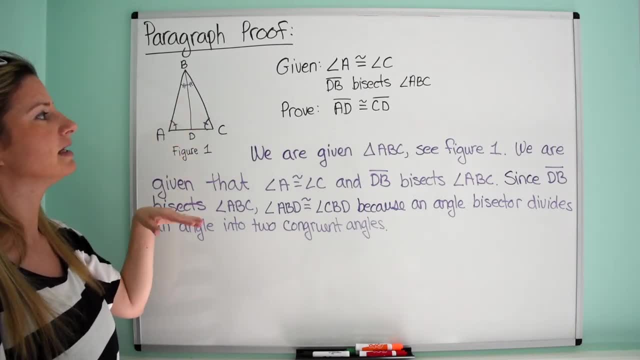 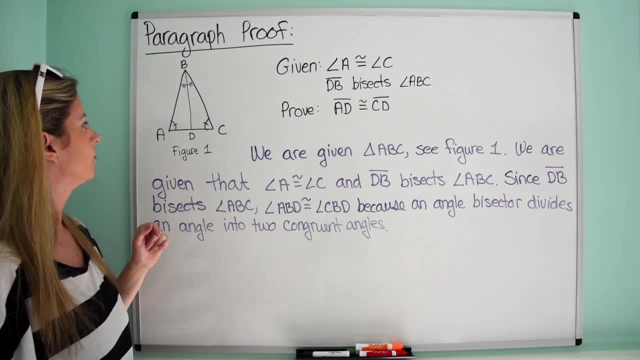 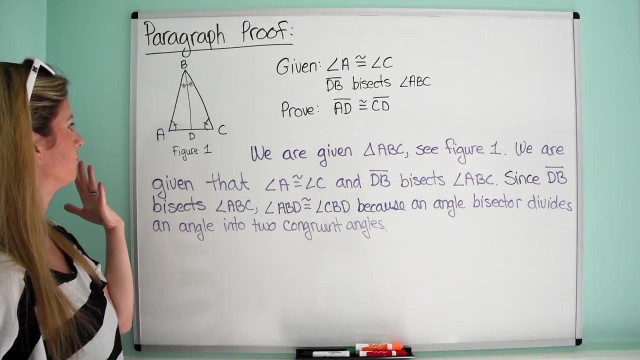 these two triangles are congruent. we can then use CPCTC to prove that the corresponding parts of the congruent triangles are congruent. okay, So all right. So what are we going to do next? Well, we've got, let's see, we've got two angles, but we don't have, you know, we can't do angle. 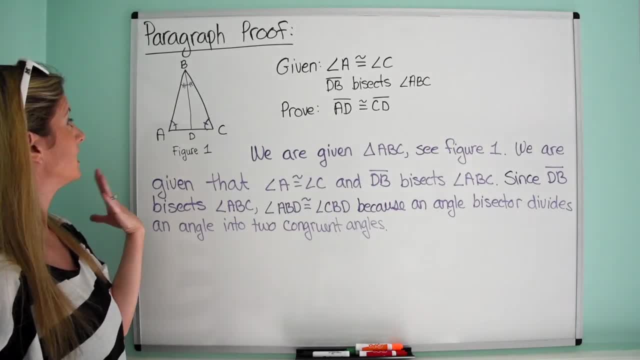 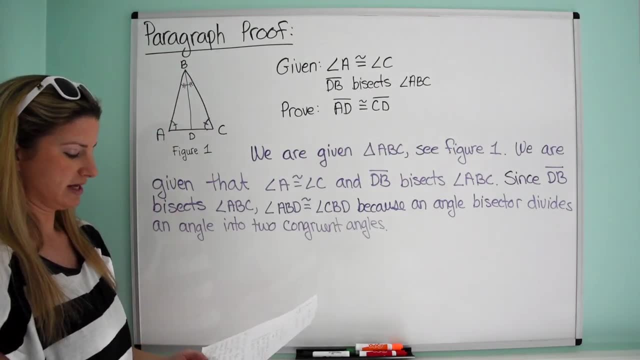 angle angle. That doesn't help. That just has similarity. So we need a side, And something we can definitely see right here is that BD is congruent to itself, So we're just going to write that out. So, instead of writing BD is congruent to BD and then reason reflexive property, we're 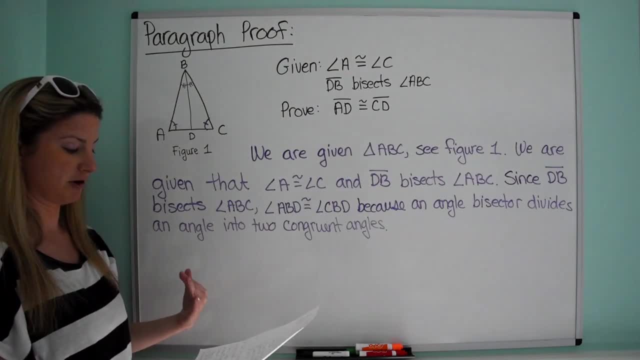 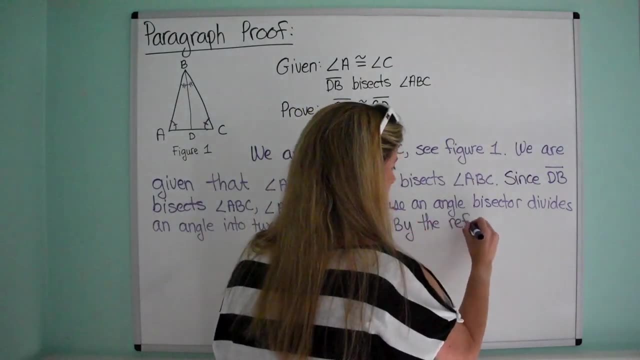 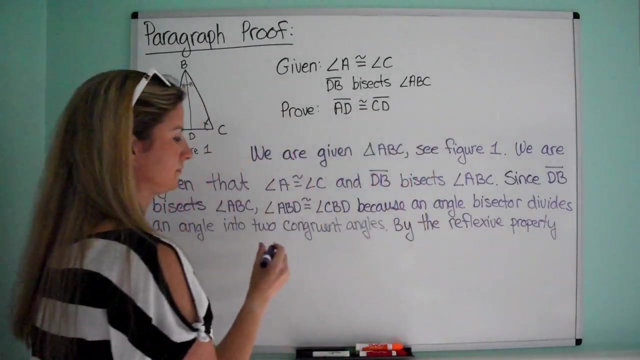 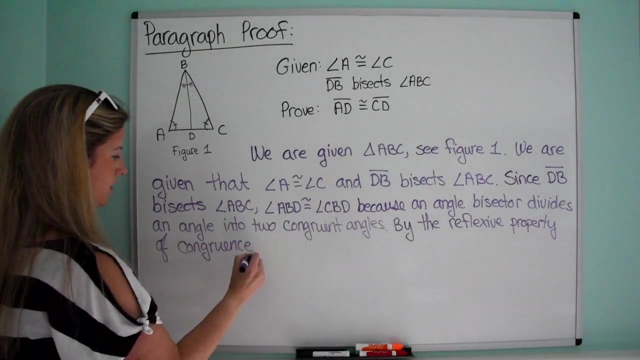 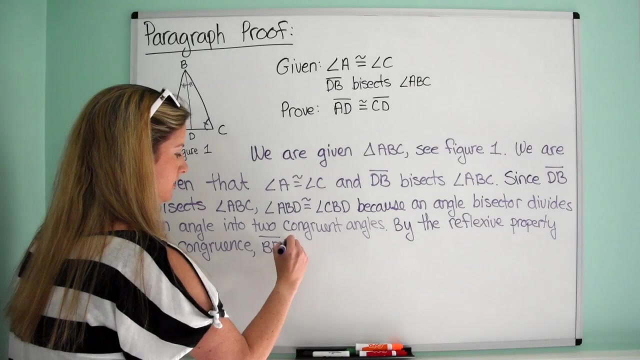 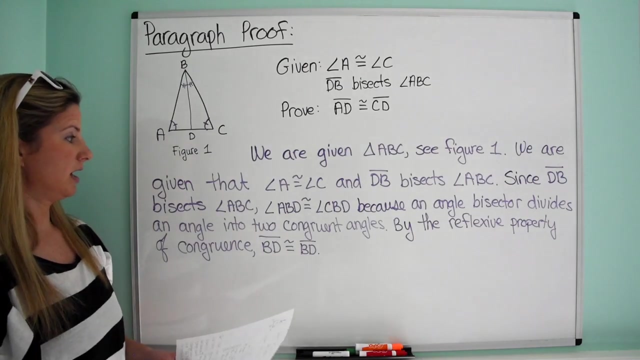 going to write it in a sentence. So the reflexive property of congruence, comma: okay, BD is congruent to BD. Segment BD is congruent to BD, Okay, Perfect, All right, So now we can write that up. All right, So now we know that these: 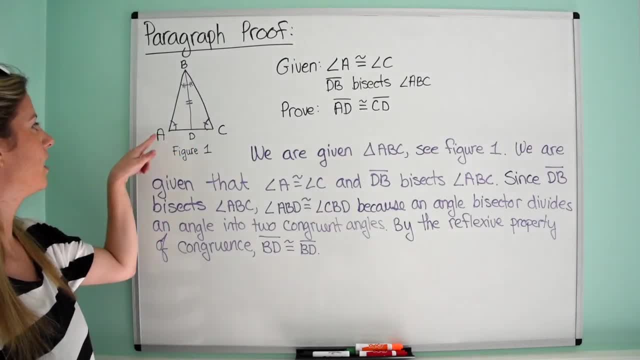 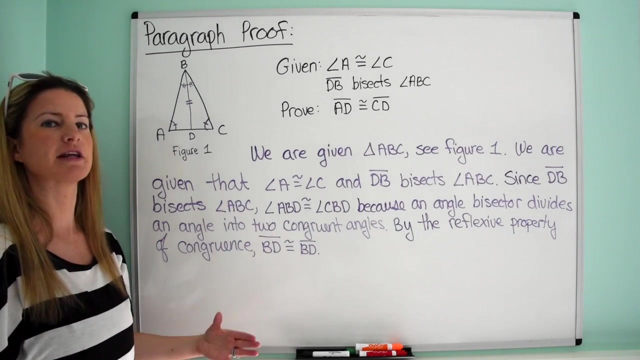 two triangles are congruent, So triangle ABD is congruent to triangle CBD by angle, angle side. Okay, So we just need to write that out. So then here's where it gets kind of. we kind of have to list everything before we write this out, okay. 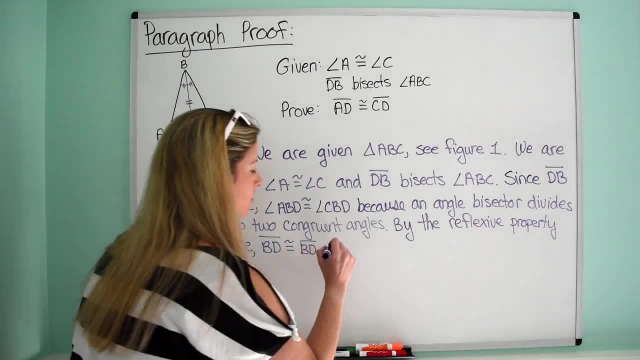 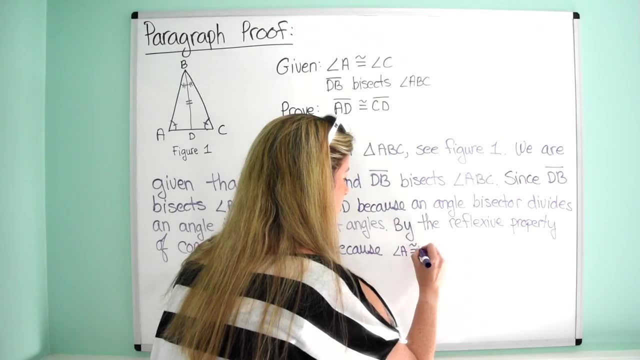 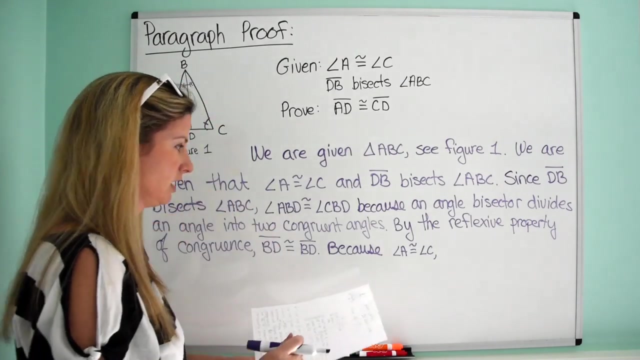 So we have to say, because we're going to start with because, Okay, So, because angle A is congruent to angle C, Okay, So, boom, boom, Okay. Then the next thing was that these two angles were congruent. So angle ABD is congruent to angle CBD. 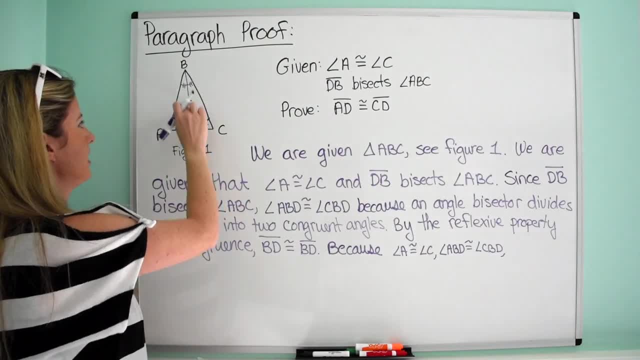 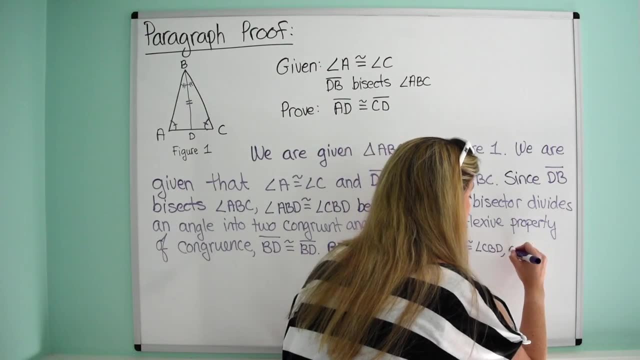 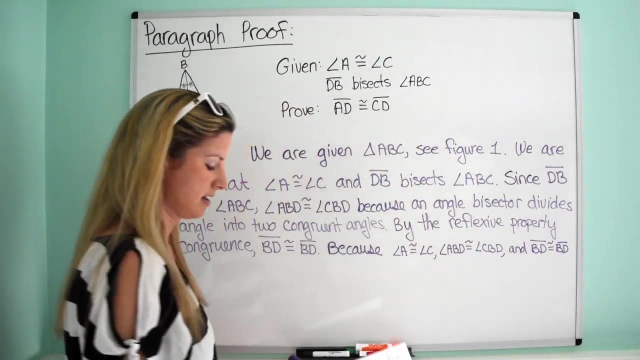 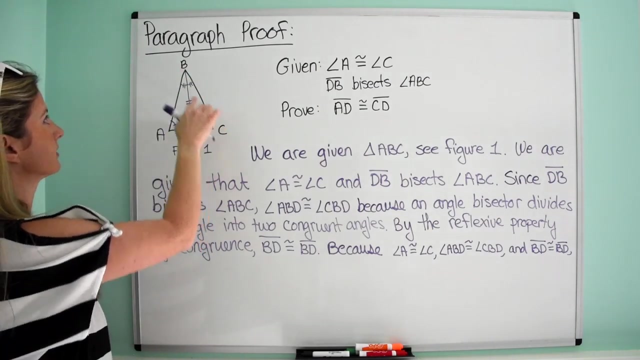 Okay, care of this and these two. and the last thing was what we just said, which was: and BD is congruent to itself. okay, then we get to the two triangles. so triangle ABD is congruent to triangle CBD. okay, so triangle ABD is congruent to. 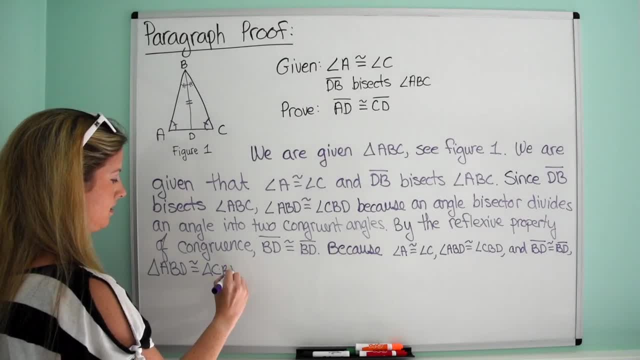 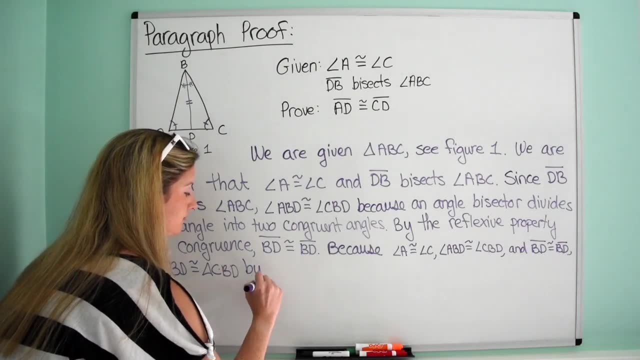 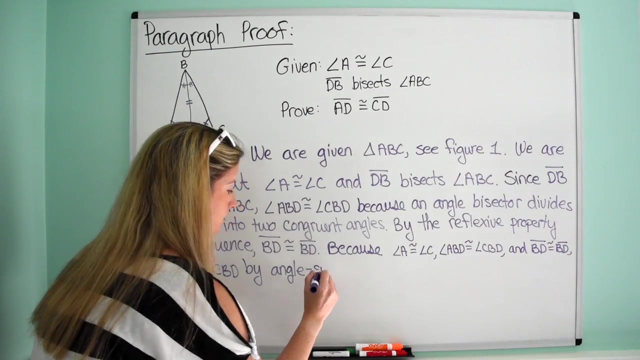 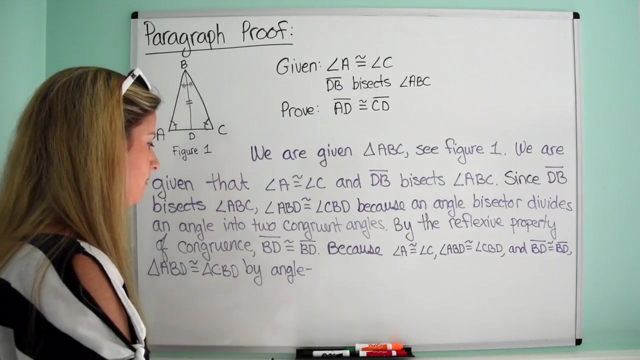 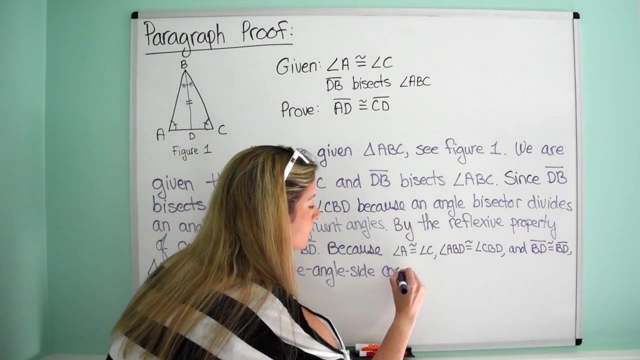 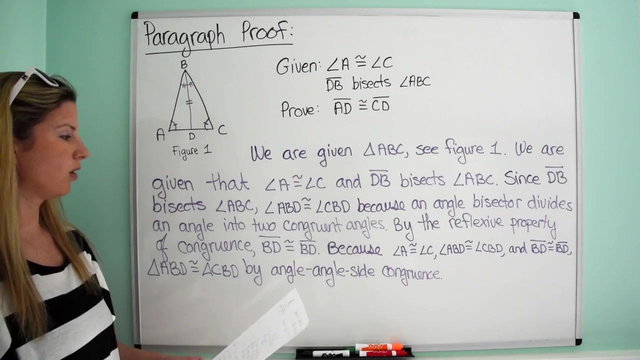 triangle, CBD, okay, and then here's where we get. here's where we have to actually write it out by angle. okay, and I just do dashes, oops, not side, it's angle, angle, side, angle, angle, side, congruence, okay, all right, so you know what? and we probably should write angle. 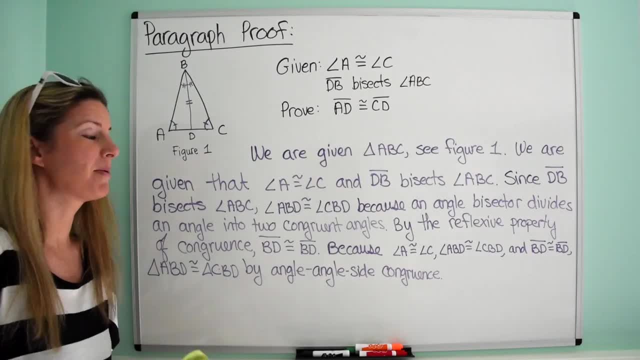 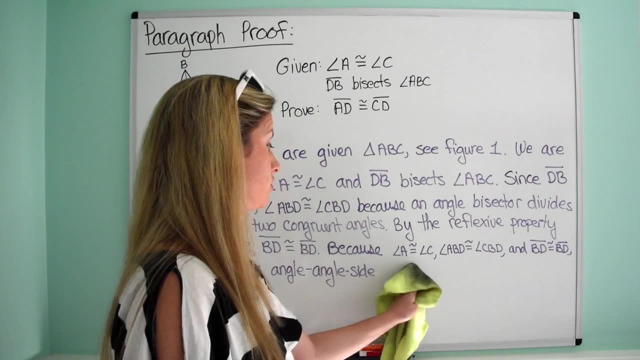 angle side triangle congruence. and again remember I said you just you need to check with your teacher and see how specific they're gonna be, because some teachers are gonna be really specific and say you needed that triangle congruence in there. some teachers are gonna be a little laid-back, some may not. 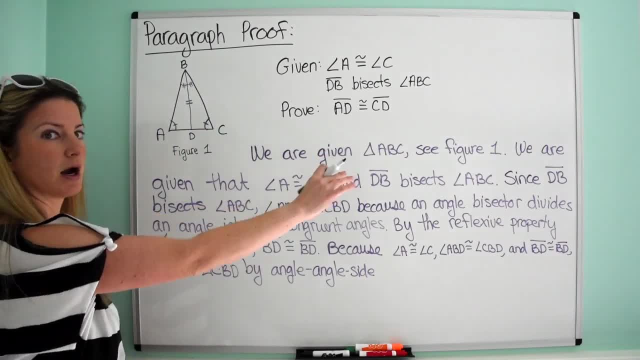 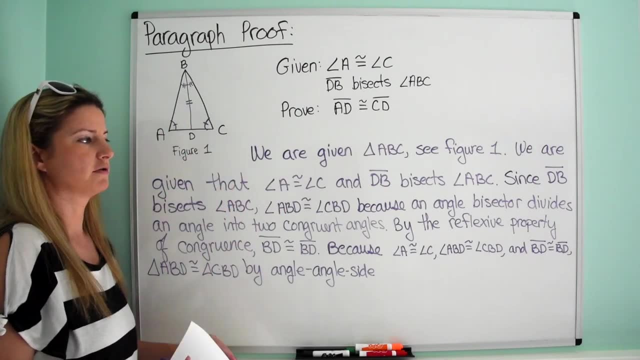 make you write this whole thing out because you've already listed everything up here. so that's where checking with your teacher with two column proofs there's kind of like really like this is how you do it with paragraph proofs, there's like a lot more leeway. so that's where I think that's why a lot of teachers do. 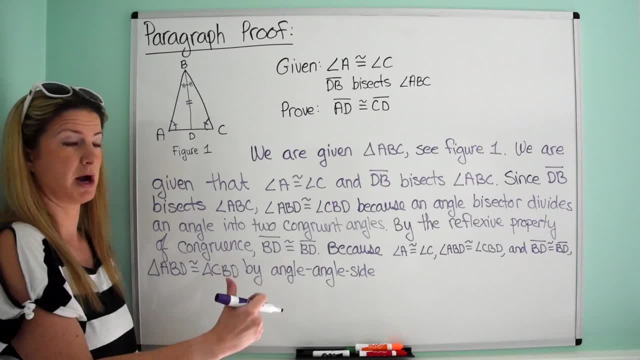 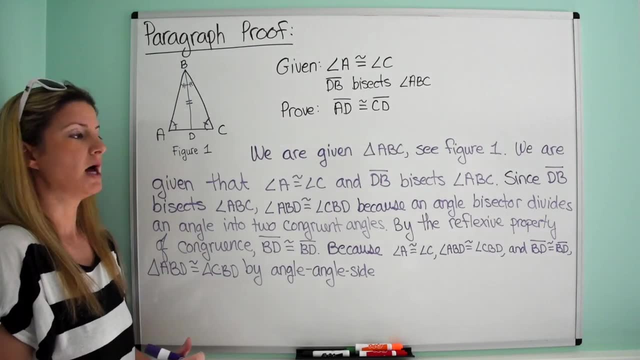 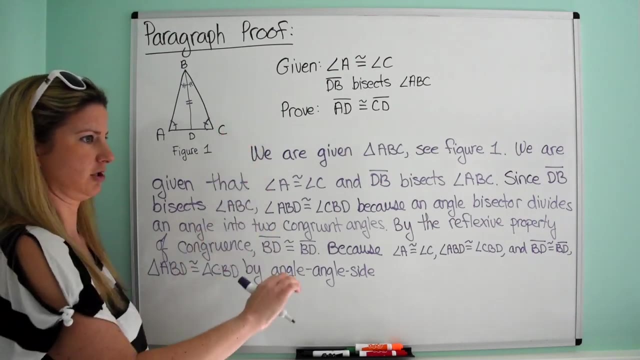 stick to two column proofs. I taught all, I taught paragraph, I taught flow and I told the kids on on a test, you can do any proof you want, flow paragraph or two column. but I then started to work mainly with two column, just because I think it's it's more concise. you just get to your point. here's what I can do and 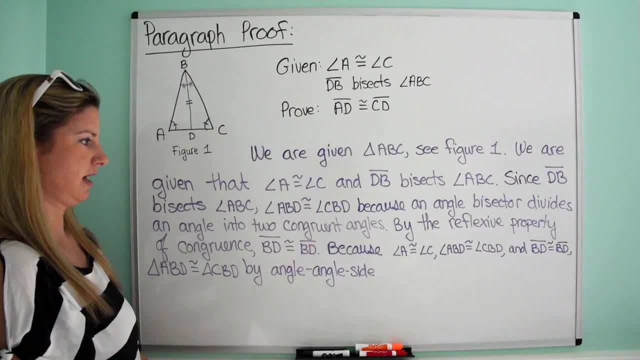 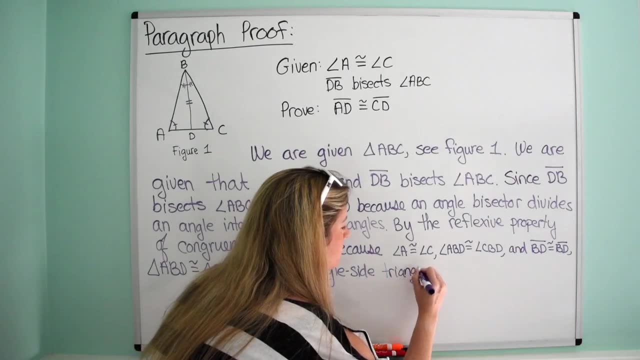 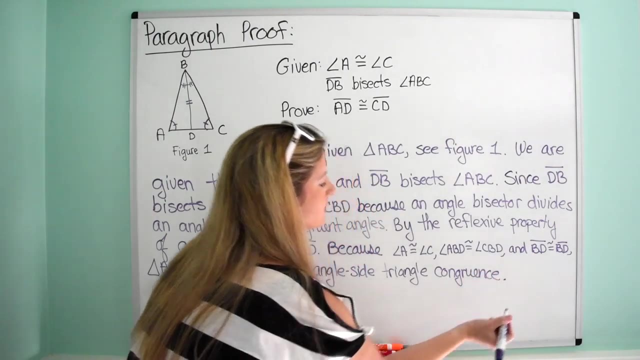 this is why we don't get worried about all the words and how we list it. okay, so by angle, angle, side, triangle, congruence. okay, so we are almost done. did I spell that right? congruence, okay, perfect, so now we're to our final step, so we 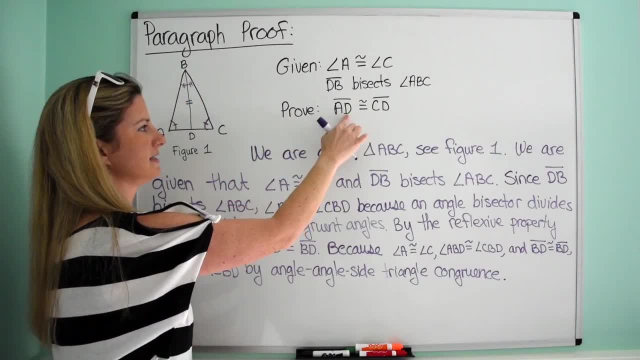 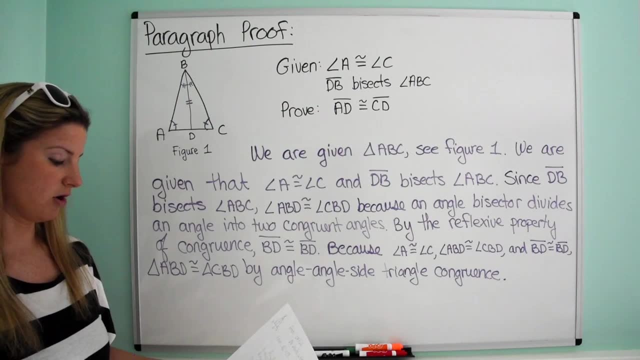 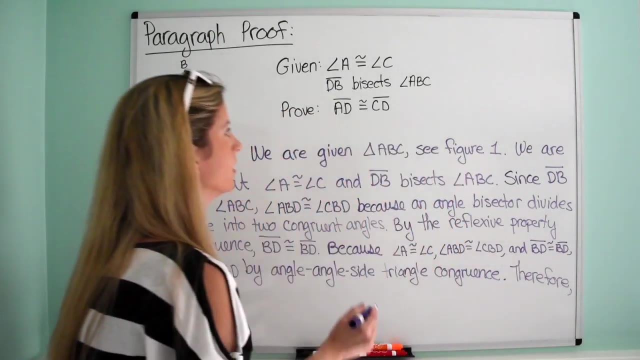 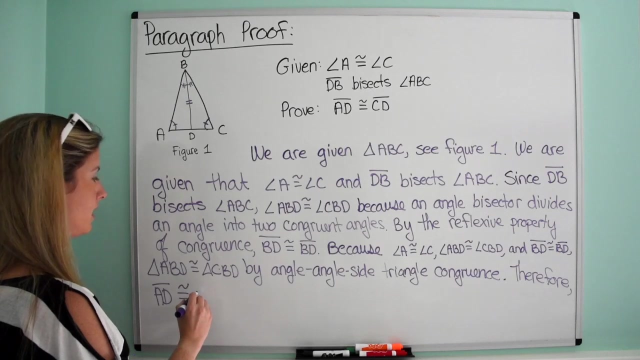 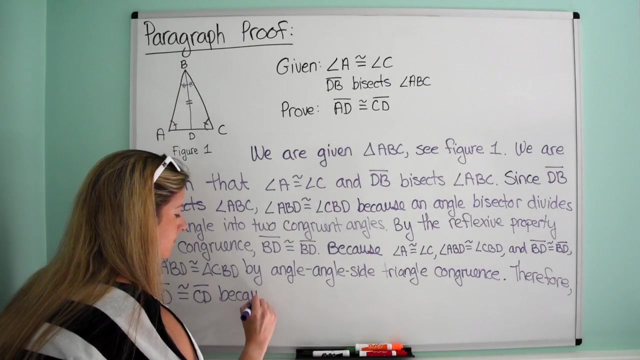 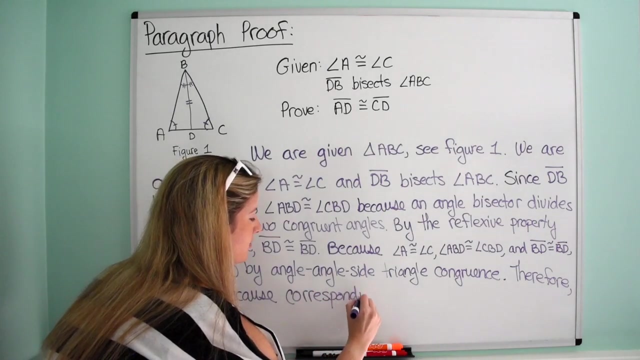 prove these two triangles are congruent. so now we know that AD is congruent to CD by CPCTC. so now we just have to kind of write that out, okay. so we write therefore, okay, and then write what we're proving: so AD segment AD is congruent to segment CD. okay, because corresponding kind of check my 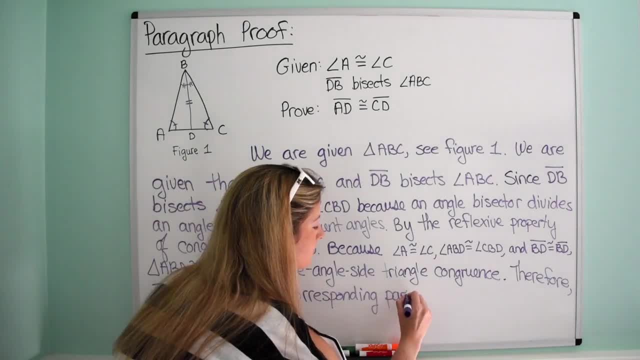 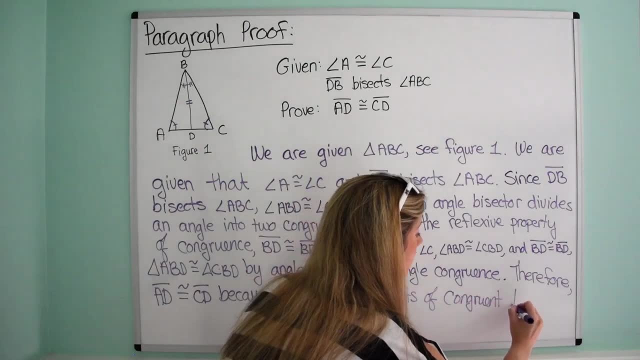 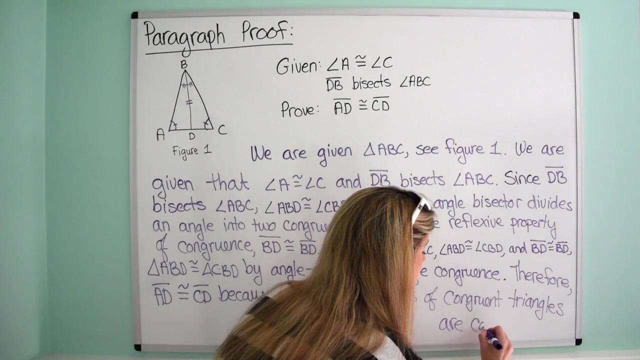 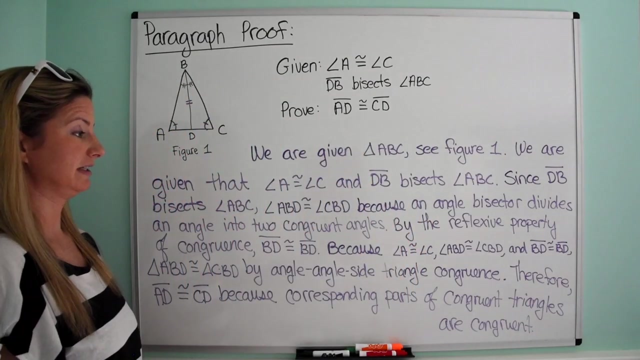 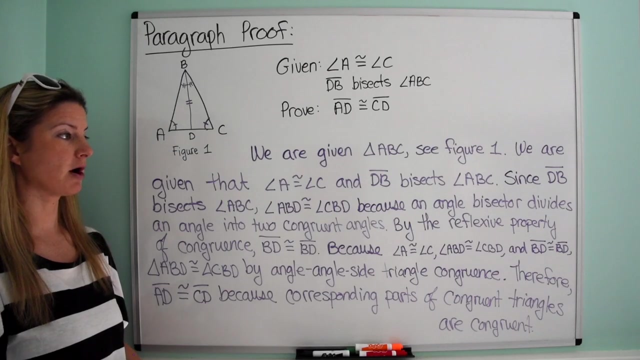 spelling here. corresponding parts of congruent triangles- almost out of space here- are congruent. I'll just write it down here. perfect, and that's it. we proved it. so here's an example of a paragraph proof. um, now, every teacher is different. some teachers might really like paragraph proofs, but I'm not.